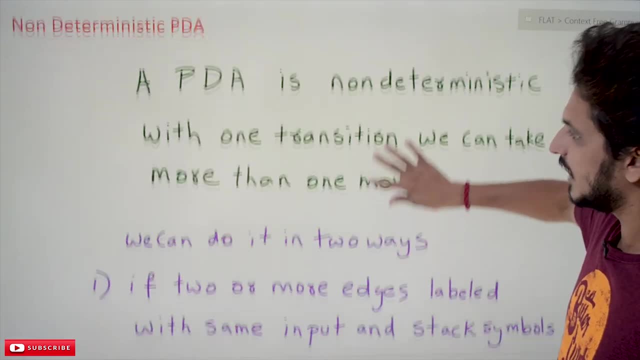 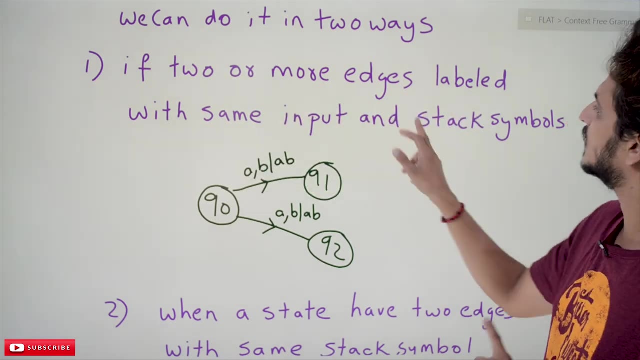 Then we can say it is non-deterministic pushdown automata. We can do it in two ways. What's the first way is if two or more edges labeled with same input and stack symbol. Let's take an example On Q0, the input symbol is A and the stack top is B. 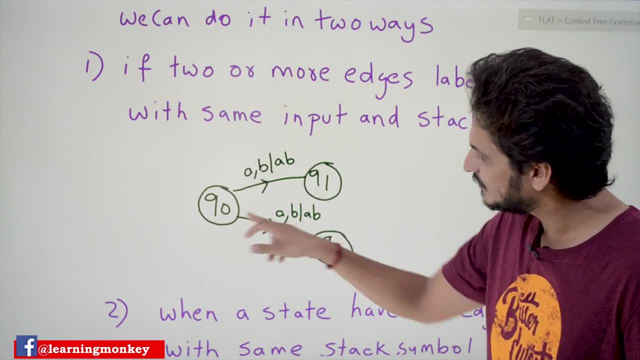 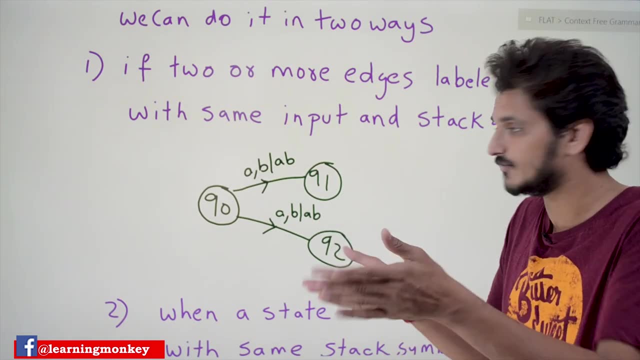 We are doing some operation and moving to Q1.. The same thing: input symbol is A and the stack top is B. We are moving to Q2.. This we call it as we are moving to two different for the same input and stack symbol. We are moving to two different states That we call. 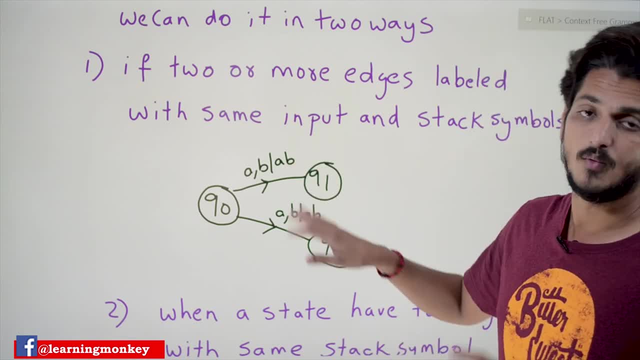 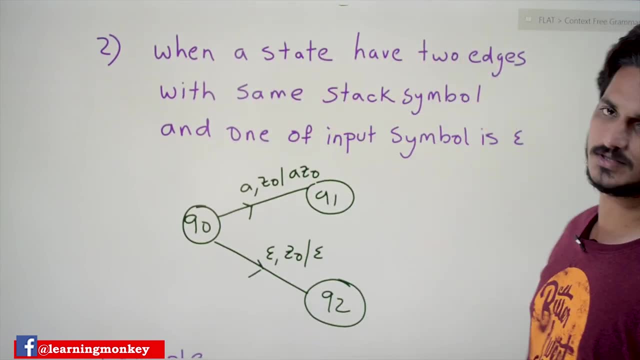 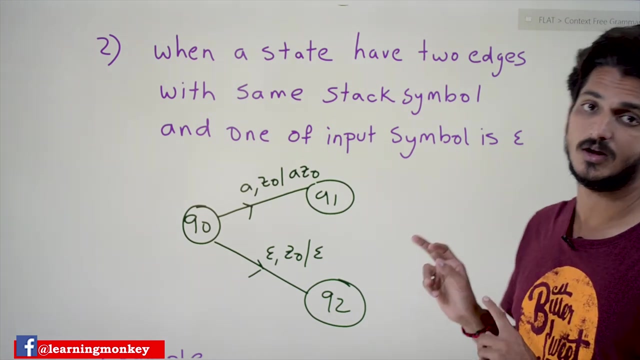 it as a non-determinism. This is one of the way We are having other possibility also. What's that possibility is when a state have two edges. if a state is having two edges with same stack symbol and one of input symbol is epsilon, One of the input symbol should. 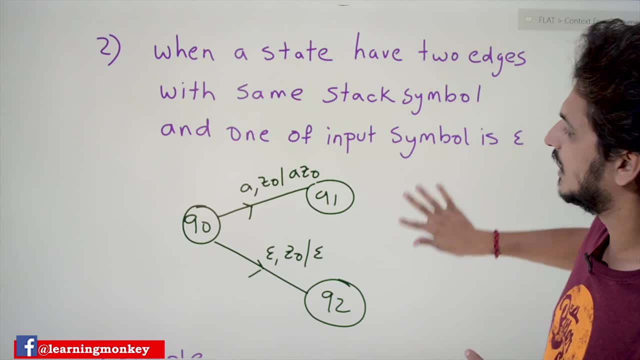 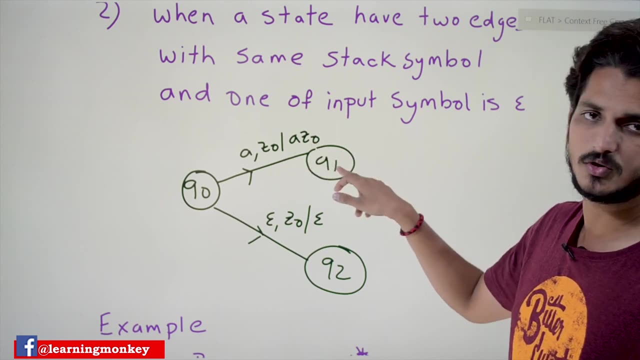 be epsilon and it should have the same stack symbol. What's the example On Q0, if you take the input symbol is A and stack top is Z, we are doing some operation. and moving to Q1.. If you take the input symbol is epsilon and the stack top is Z, we are doing some. 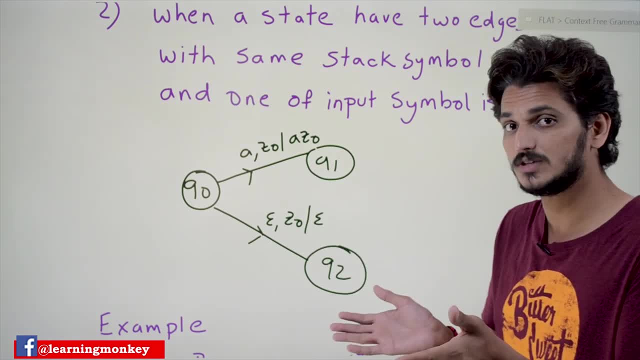 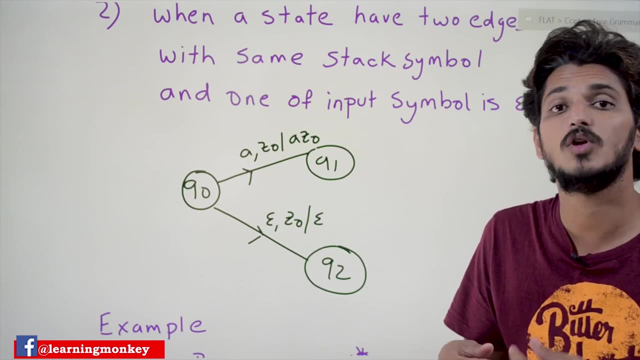 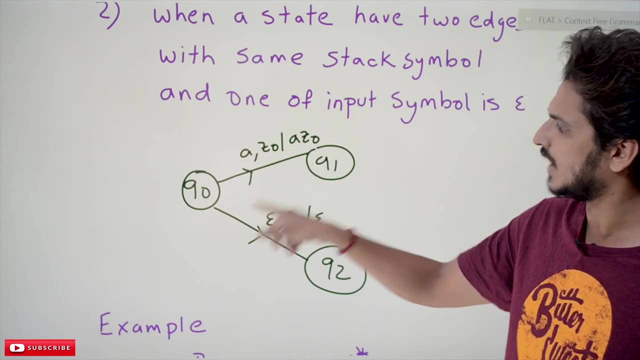 operation and moving to Q2.. Here also we are moving to two different states. But stack symbols are same, but input symbols. one of them is epsilon Means. using epsilon we can move. Epsilon moves transactions. One is by taking the input symbol A we are moving. Other is by taking epsilon Means. we can move without taking. 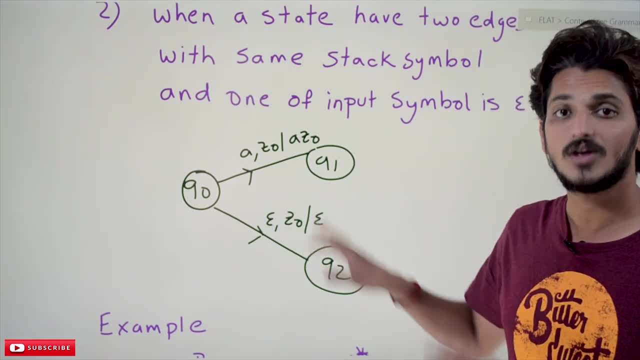 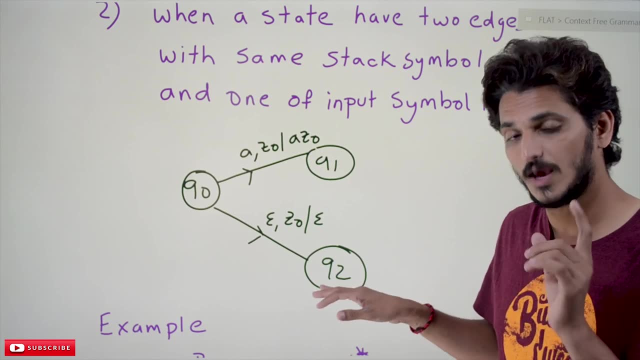 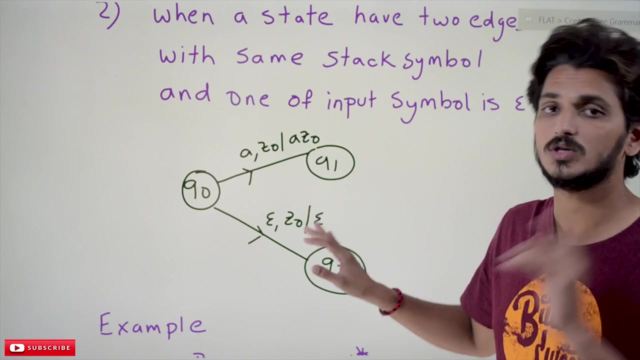 the input. also, we can move to Q2 state. This also considered as non-determinism in pushdown automata. Hope you understand, because if you don't know what's epsilon moves and what non-deterministic epsilon moves in finite automata, it's unable to understand this concept. Please watch those. 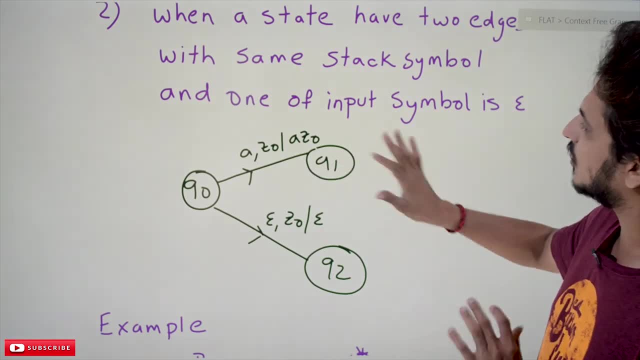 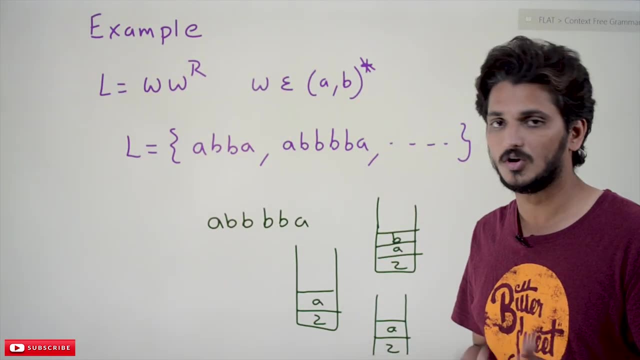 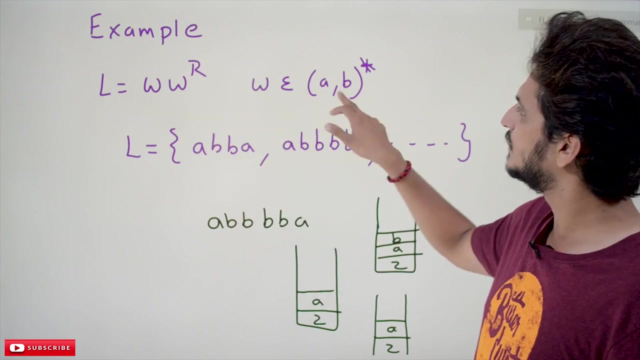 classes and compare. So this is how we provide non-determinism in pushdown automata. Let's take an example and understand how we write the non-deterministic pushdown automata for the given language. Let's take: L is equal to W, W power R. where W belongs to A or B, whole star Means you. 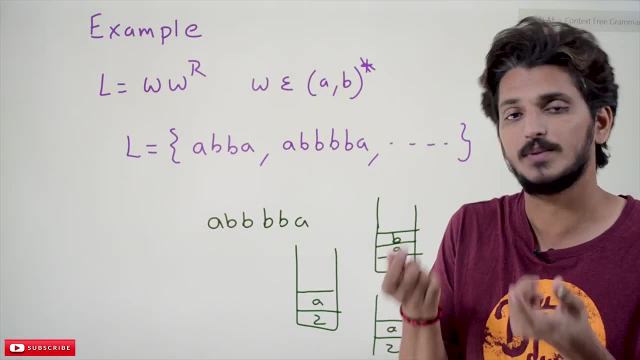 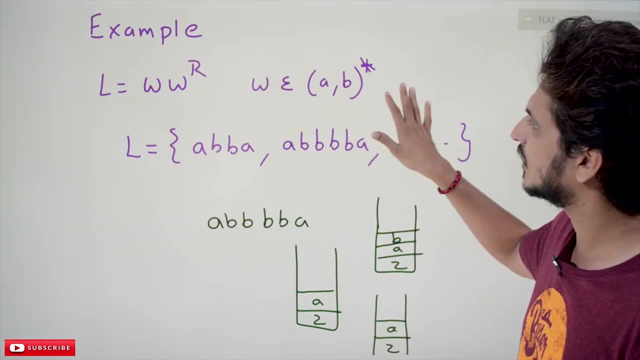 take any string that belongs to A plus B whole star. A plus B whole star means the strings that are generated using A plus B whole star. any string can be accepted. Okay, so if you take the inputs, L is equal to W, W, power, R. These type of string should: 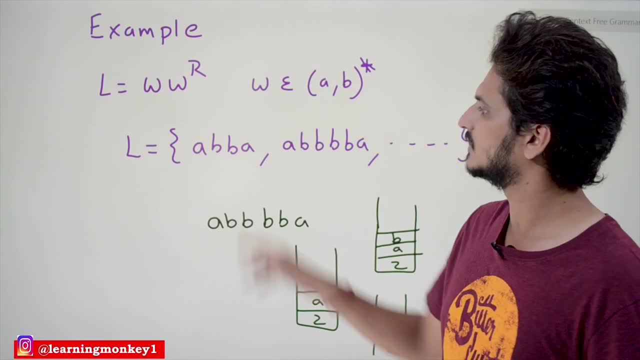 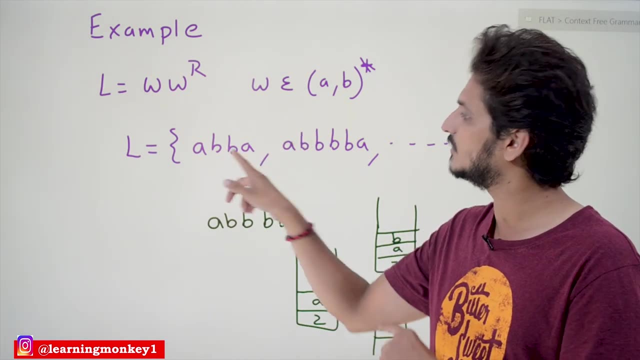 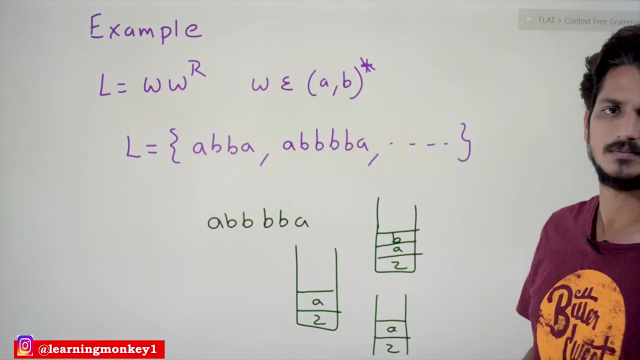 be accepted. L is equal to ABBA. Yes, AB, if you consider it as AB, as W, and BA means W, power, R Reverse of AB means BA. This is accepted. ABB BBA. Yes, this is accepted. Okay, ABB BBA. 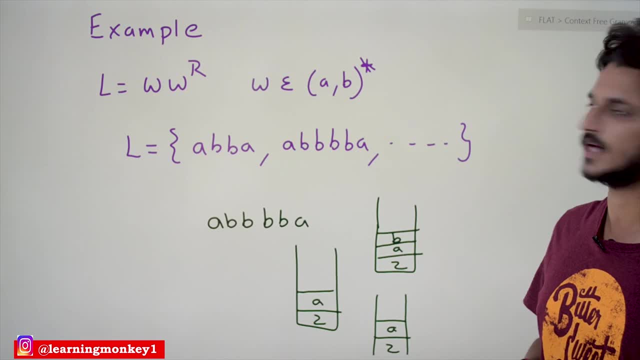 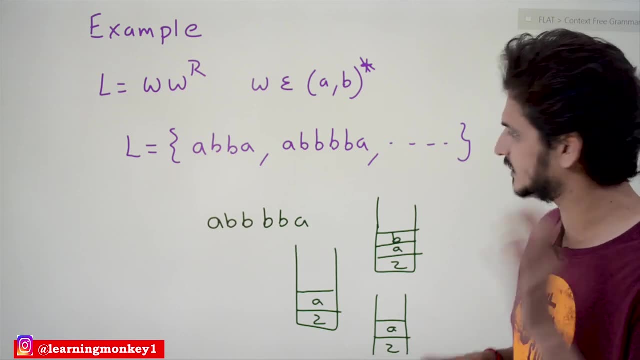 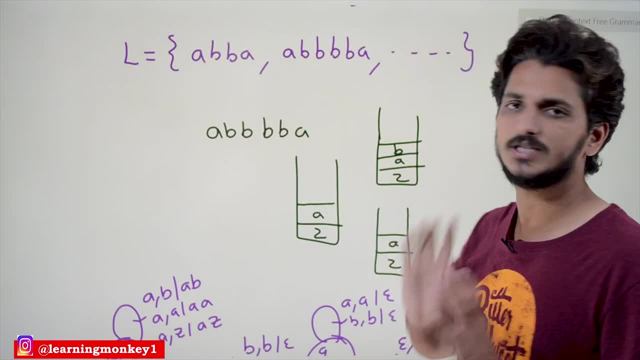 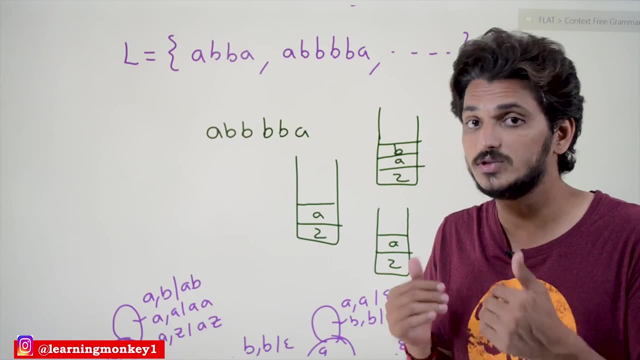 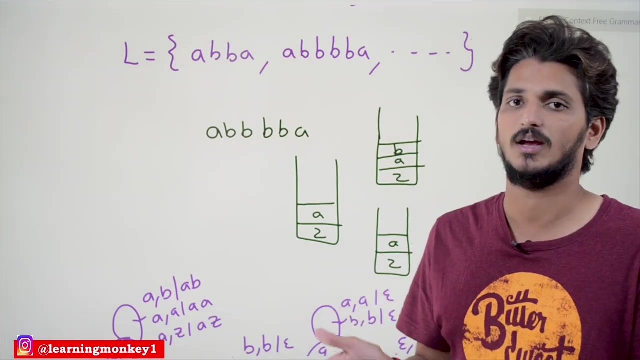 is, whenever you see the first input symbol, push on to the stack. If you see the second input symbol, we have to check for two conditions. So why we have to check for two conditions? We think that because here we don't know which. where is the middle of the string? 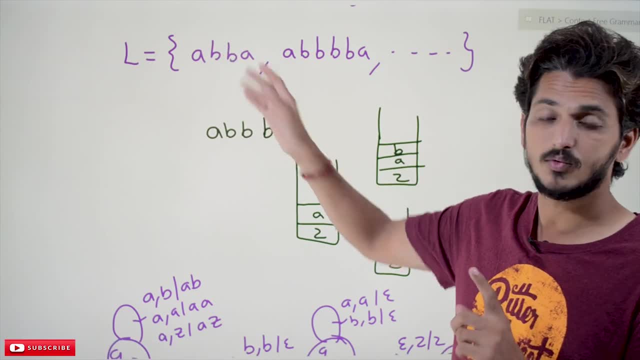 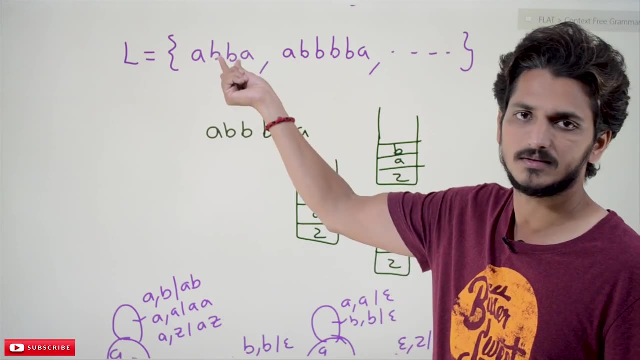 See, here we have to identify two logics: A, B. After that we have to check for pop operation. If you see B, B, pop Means there is a matching. A A- Yes, there is a matching. 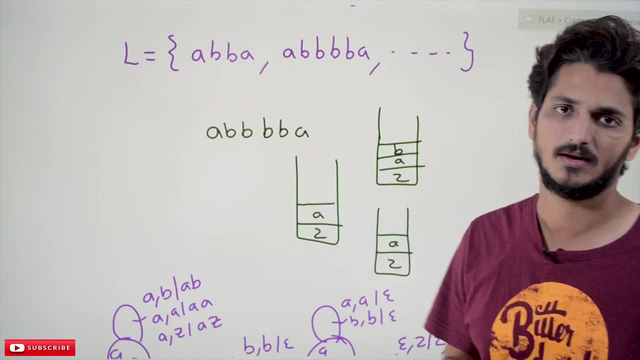 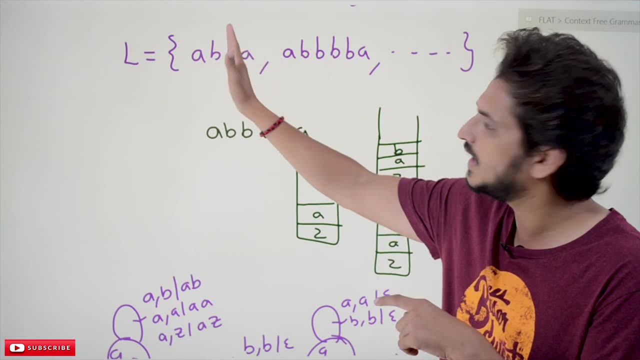 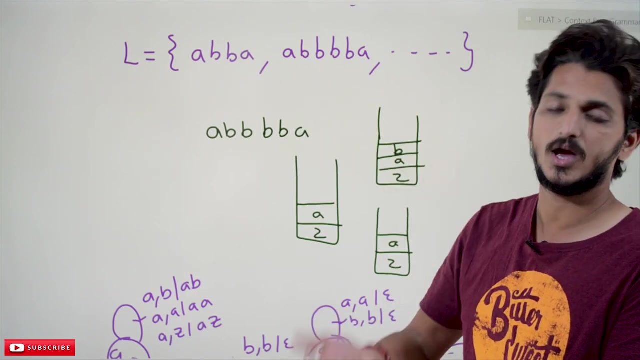 Exactly reverse of W is happened here. Exactly reverse of W is happened here. So that's why it is accepted. Means from the middle. we have to check for pop logic. If you see B and stack top is B, we have to pull it. 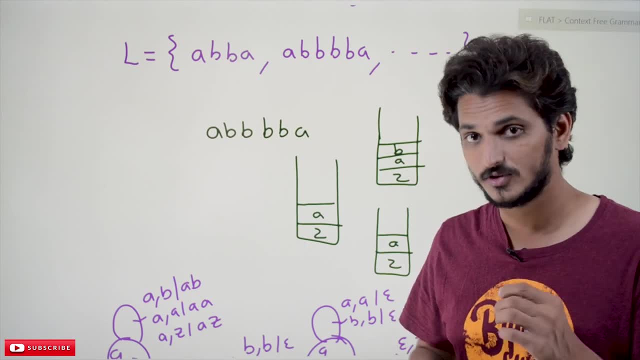 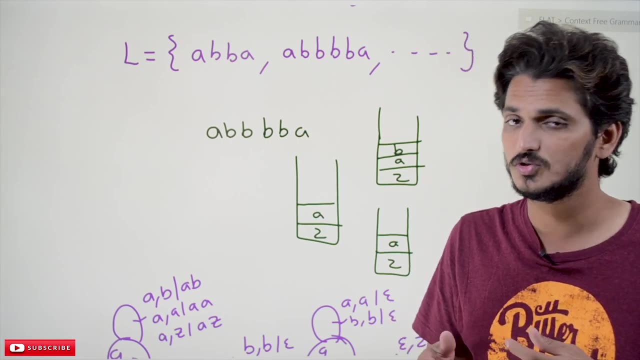 We have to pop the operation. But the confusion is: where is the middle of the string? We don't know what's the middle of the string. That's why we are using the non-deterministic pushdown automata. We think that from the second symbol onwards what we have to do. 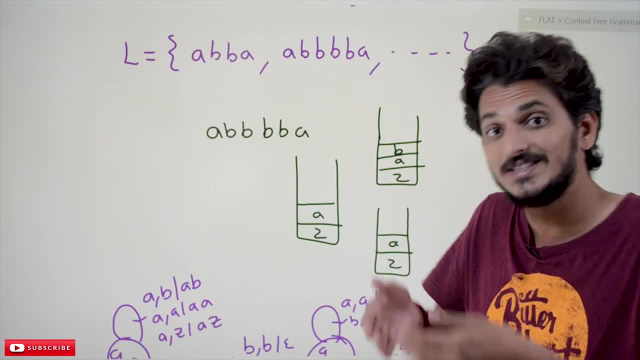 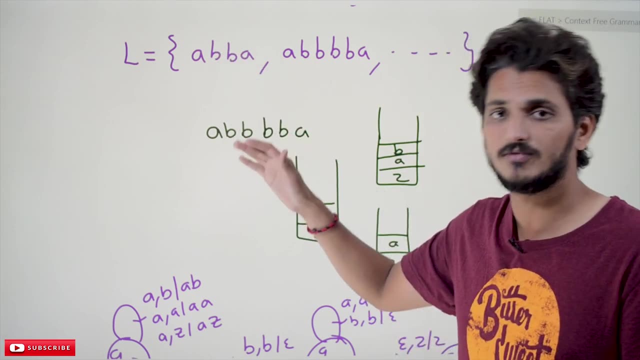 We have to consider it as each time. we consider it as this is the middle of the string. From second symbol onwards: this is the middle of the string. Yes, third symbol: assume that this is the middle of the string. Assume that the next symbol, this is the middle of the string. 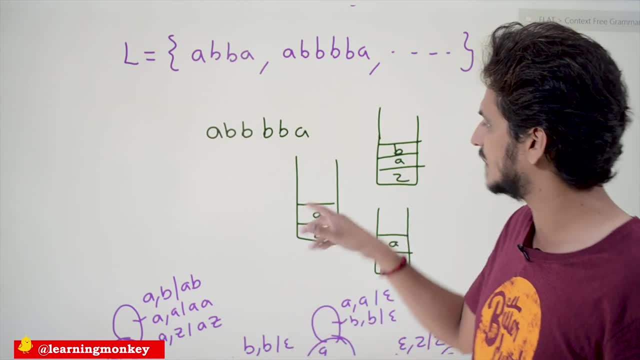 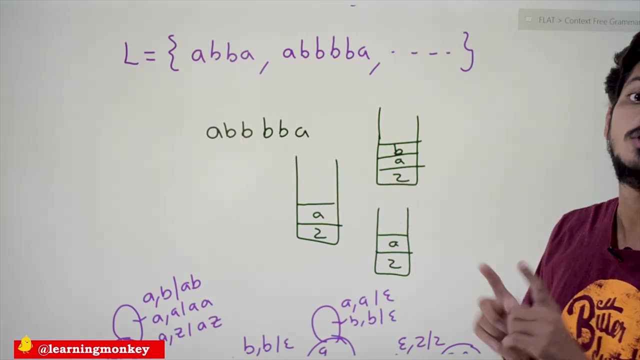 Based on that logic, we will move to two different states. See here for the first input symbol A, we have pushed on to the stack. From the second input symbol B, we are doing two operations. One operation is push operation, Assuming that this is not the middle of the string. 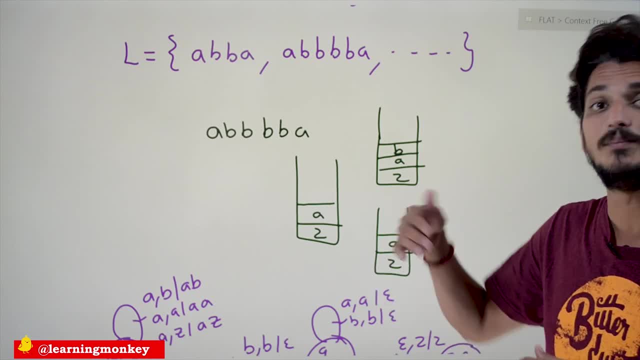 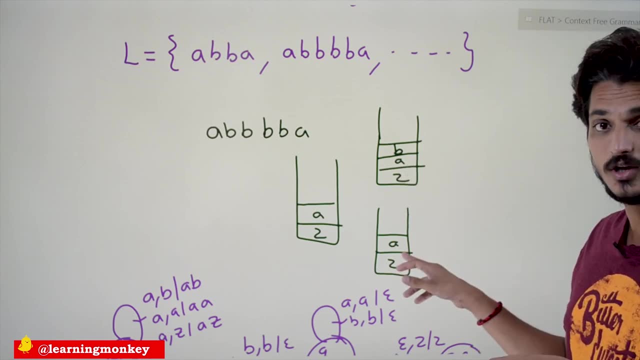 Second operation is pop operation. Assuming that this is the middle of the string Means we are taking. One pushdown automata is going to check the push logic. Other pushdown automata is going to check the pop logic. Reverse of the string- pop logic. 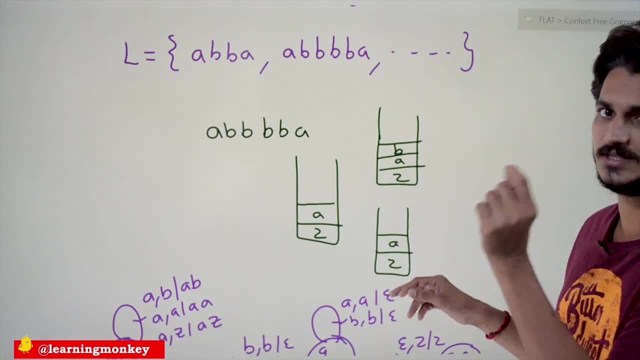 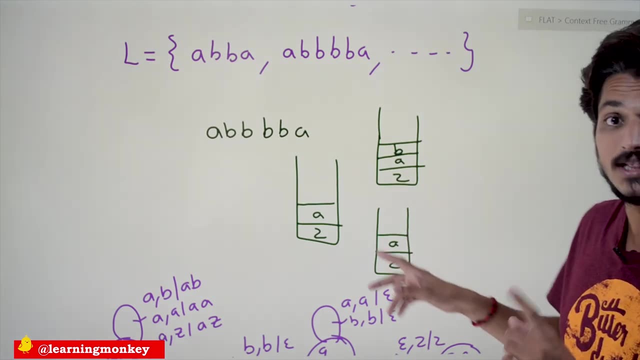 This example we already discussed previously With C example. Please watch that example and come back here. That's why we said that please watch our previous class and come back here. So in the final, at least one of the pushdown automata is going to succeed. 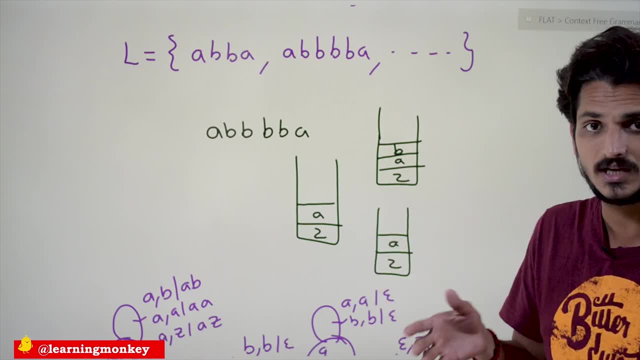 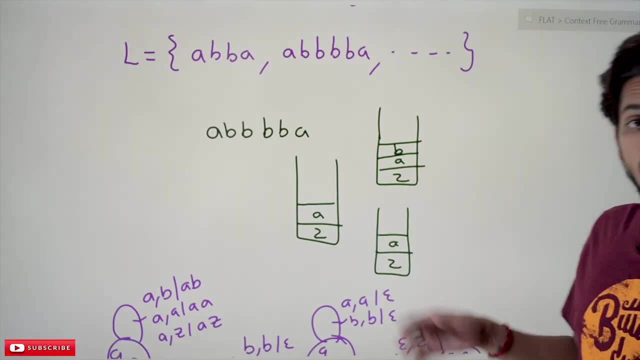 That's why, because each time one machine is going to identify that we have to push, this is not the middle of the string, so push it. One machine is going to check the logic. That is, assume that this is the middle of the string and try to check the pop logic. 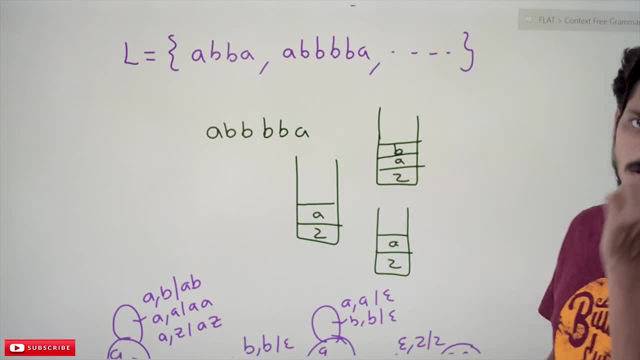 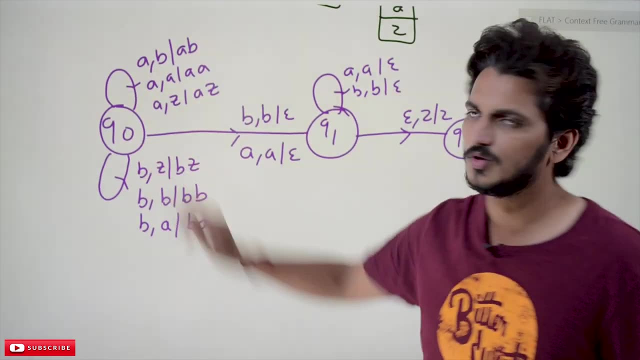 That is how we write the pushdown automata- non-deterministic pushdown automata for the given language: W, W, power, R. How we write that On Q naught. this is the starting of the starting state On Q naught. if you take A. 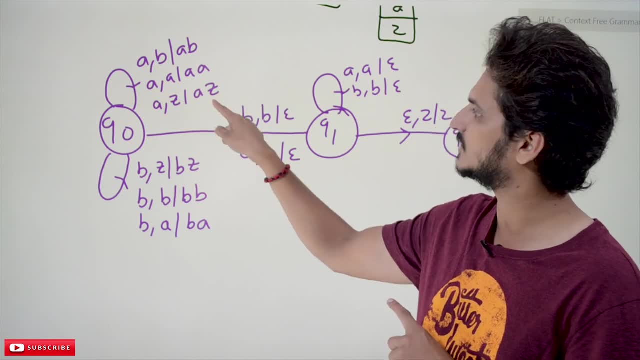 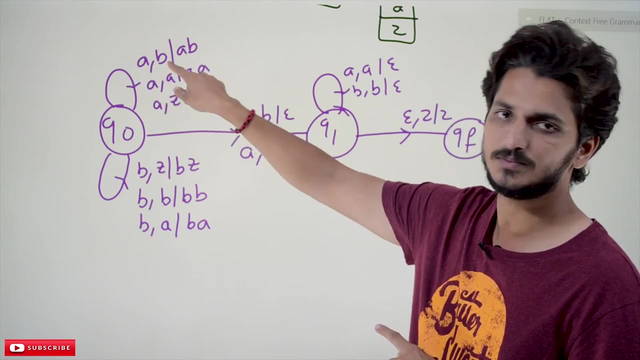 the. if you take A and stack top is Z: yes, push. If you take A and stack top is A: yes push. If you take A, input symbol is A and stack top is B: yes push. If the input symbol is B, stack top is Z: yes, push. 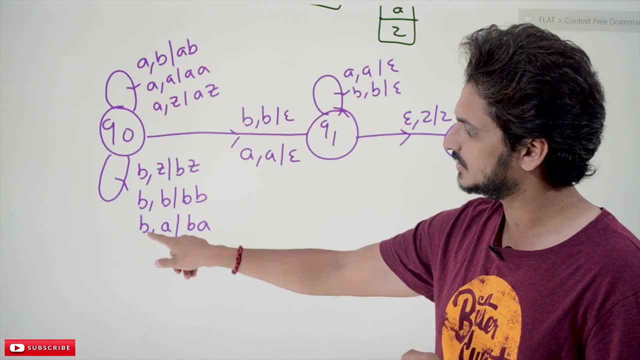 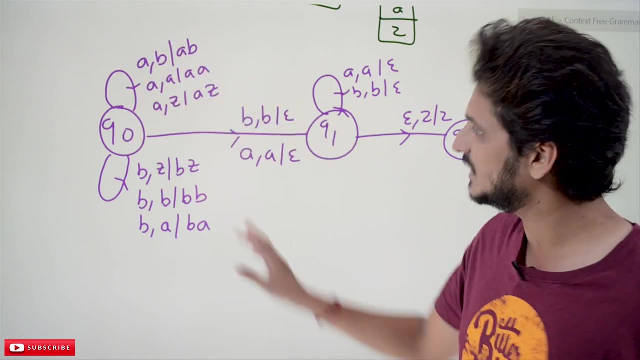 Input symbol is B. stack top is B. push Input symbol is B. stack top is A. push on to the stack. This is a. all the possibilities has been written. Whatever you see here, push on to the stack, But where we are writing the pop logic. 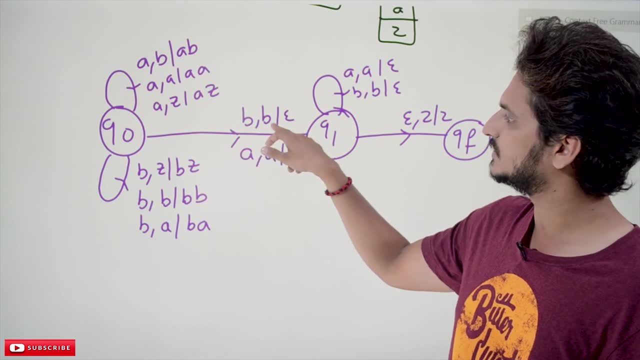 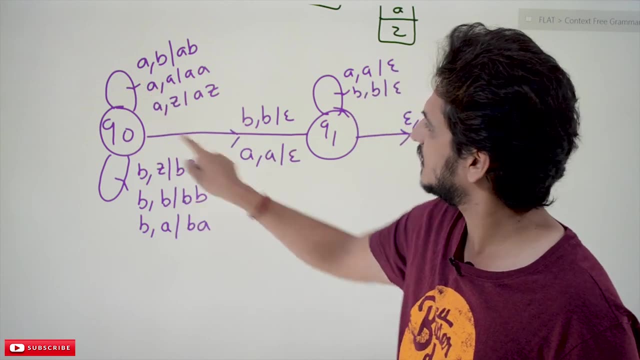 whenever you see the input symbol is B and stack top is B, we are popping for the same input symbol B, stack top is B. we are moving to this state. For the same. we are moving to Q 1, also.